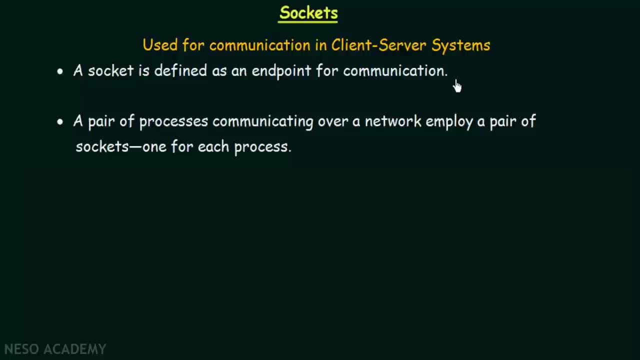 So how we can define socket is it is defined as an endpoint. So when two processes or two systems want to communicate with each other, sockets are the endpoints on either end of the communicating processes. So a pair of processes communicating over a network employ a pair of sockets, one for each process. 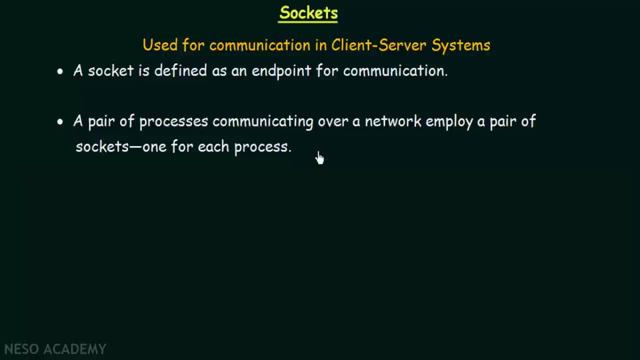 So, as I told you, when two processes want to communicate, there needs to be a connection between them, And at each end of the connection, each of these processes will employ a socket each. So a pair of communicating processes over a network will employ a pair of sockets, one for each process. 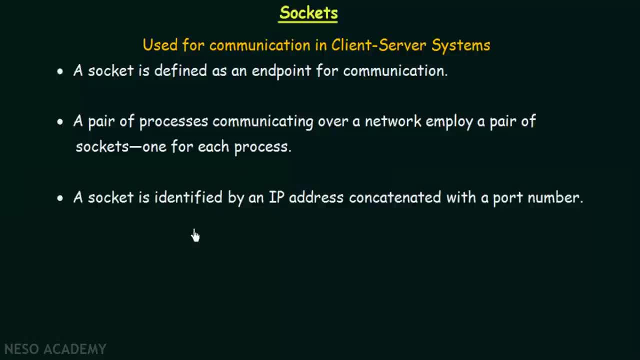 Now we will see how can we identify a socket. A socket is identified by an IP address concatenated with a port number. So a socket is identified by an IP address. Every socket will have an IP address concatenated with a port number. That means it will be followed by a port number. 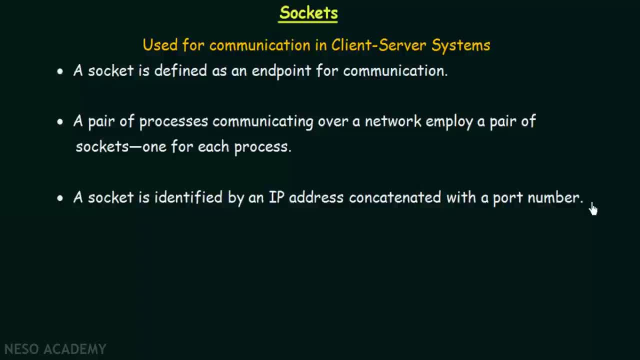 So it will have an IP address and following that, it will have a port number. So that is how sockets are identified. So I will be showing you examples of this as we move further, But for now, you remember that sockets are identified by an IP address, followed by a port number. 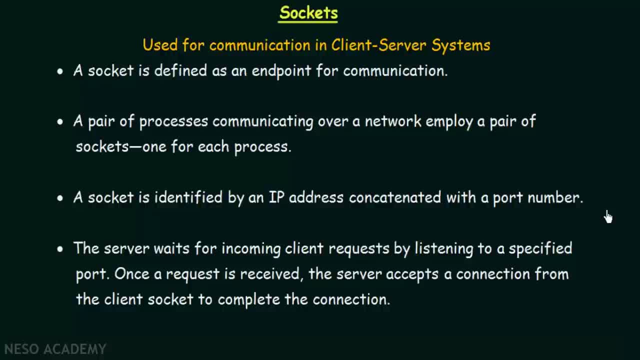 Now let us see. how does the communication between these processes employing a pair of sockets take place? So what happens is the server waits for incoming client request by listening to a specified port. Once a request is received, the server accepts a connection from the client socket to complete the connection. 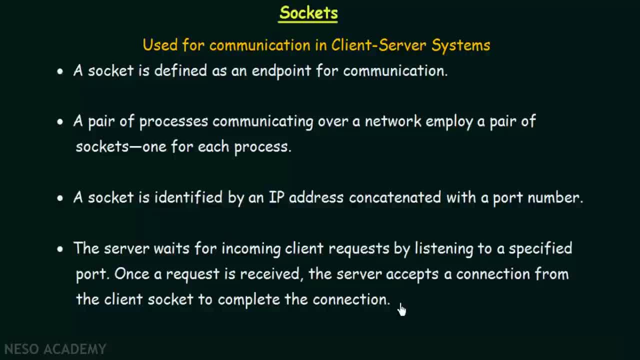 So first of all, let us understand what are client and server. You may already know, in a client-server system, the client asks for information from the server and the server will give that information to the client. That's how it works. So, in order for the client to communicate to the server and the server to communicate back to the client, 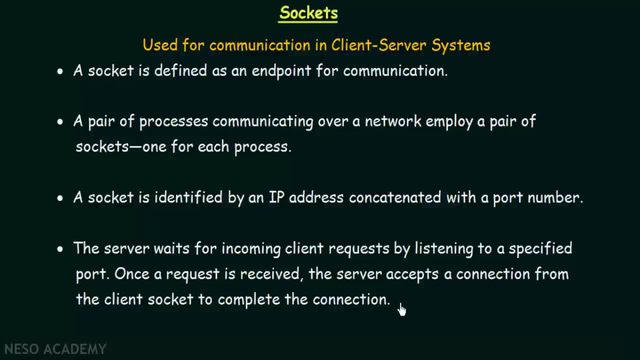 there needs to be a connection between the client and the server. So, in order to establish this connection, we are going to use the sockets And, as I told you, sockets are identified by an IP address along with a port number. So what the server does is it waits for incoming client request by listening to a specified port. 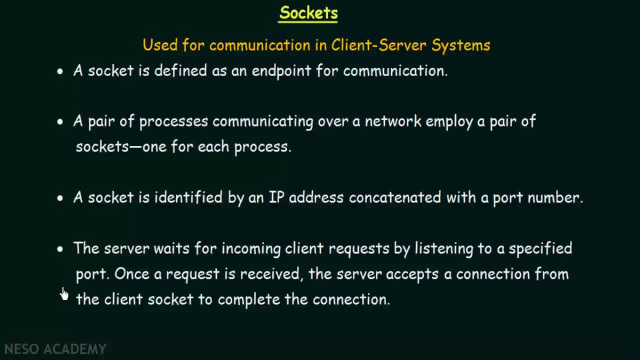 So each process will be associated with a socket and that socket will be having a port number. Now the server: it listens to the port, waiting for some incoming client request, And once a request is received, that means once a client is trying to communicate to the server. 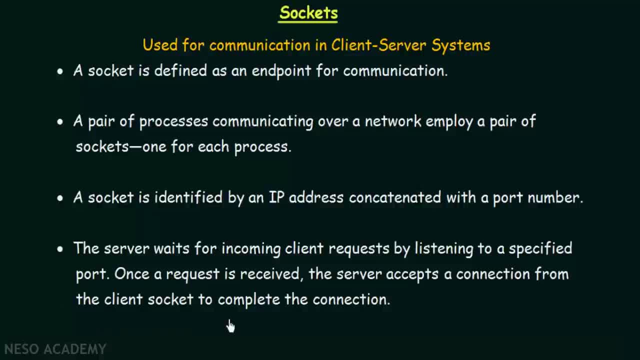 the server accepts the connection from the client socket to complete the connection. So once the server receives the connection request from the client, what it does is it will accept that connection from the client socket to complete the connection. So once a connection is established. 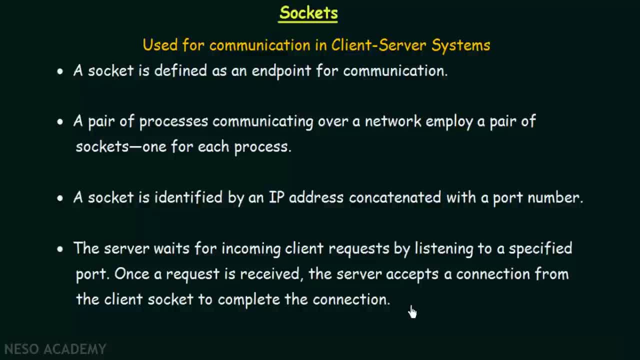 they can now communicate with the server. And remember that at either ends- at the server's end and at the client's end, with both the processes, there are sockets, And these sockets are the ones that will enable this connection to be established. 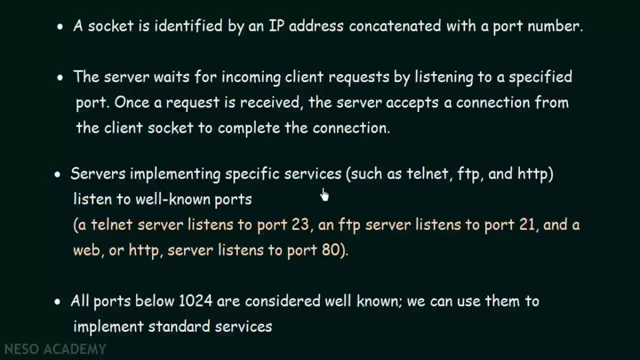 Now moving forward. servers implementing specific services, such as telnet, FTP and HTTP, listen to well-known ports. For example, a telnet server listens to port 23.. An FTP server listens to port 21.. For example, a telnet server listens to port 23.. 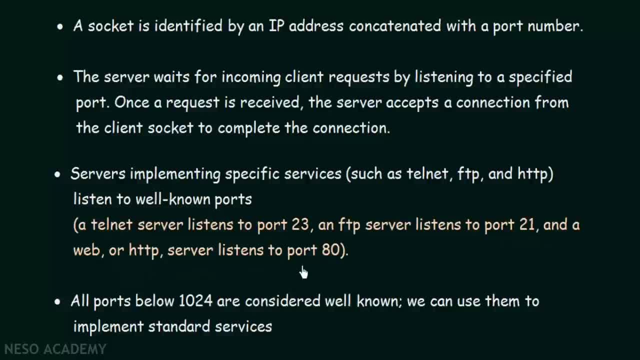 An FTP server listens to port 21.. And a web or HTTP server listens to port number 80. So, as I told you, a socket is identified by an IP address followed by a port number. So a port number is going to identify each of the processes. 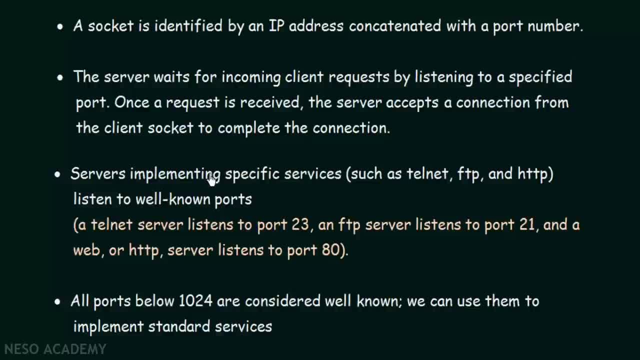 or each of the services that are going to be provided Now: servers which implement specific services, such as telnet, FTP and HTTP. these are specific services that are implemented by servers Like, for example, telnet. telnet is used for remote login. 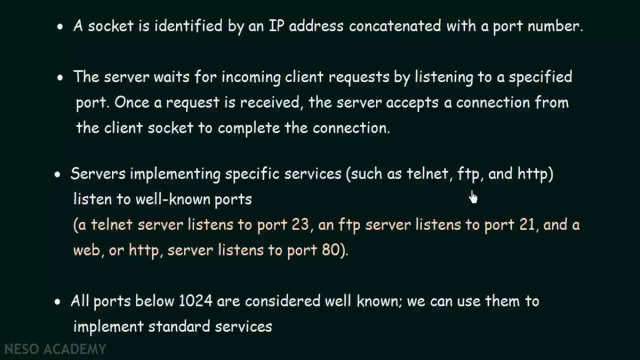 Then FTP stands for file transfer protocol, which is used for transferring files, And HTTP, as we all know, it is hypertext transfer protocol. So these are certain services that are implemented by servers, And these services, they listen to specific ports. 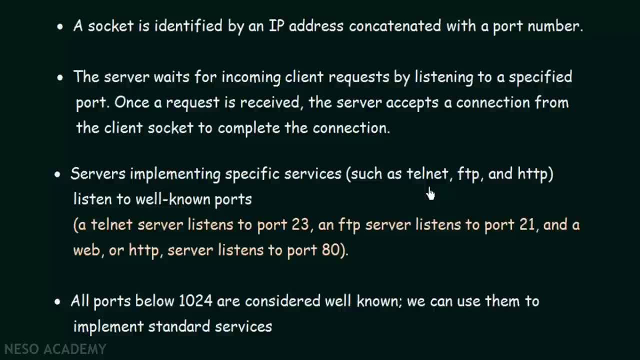 There are specific port numbers that are reserved for these specific services. So telnet, it listens to port 23.. FTP server listens to port 21.. And the HTTP server listens to port 80. So these port numbers are reserved for these specific services. 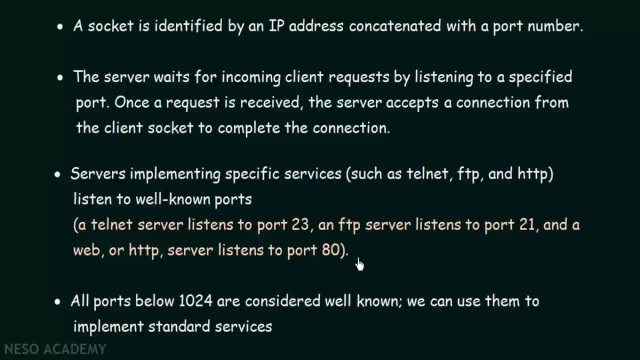 And these port numbers cannot be assigned to some other client processes or any other processes. So we should keep that in mind And it says here that all ports below 1024 are considered well-known And we can use them to implement standard services. 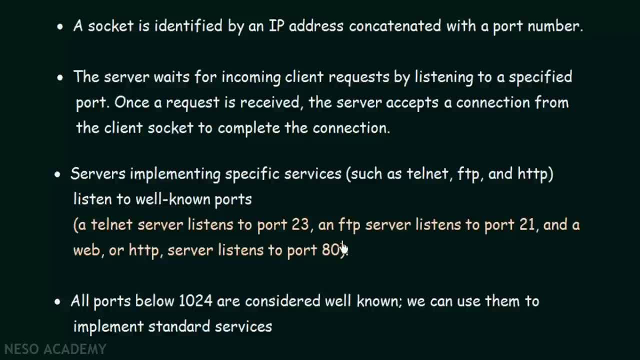 So, just like I showed you before, like telnet listens to port 23,, FTP to 21 and HTTP to 80. Similarly, all the port numbers below 1024 are reserved for specific services. Alright, so what we mean by this is. 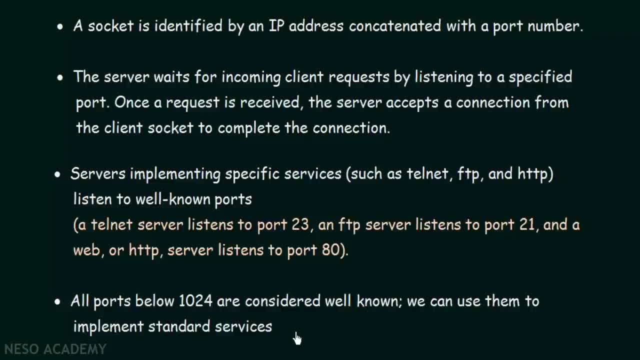 whenever we want to assign a port number to the client process or any other processes, as such, we should not use port numbers below 1024. Because most of the numbers below 1024 are reserved for standard services like the ones that I showed you before. 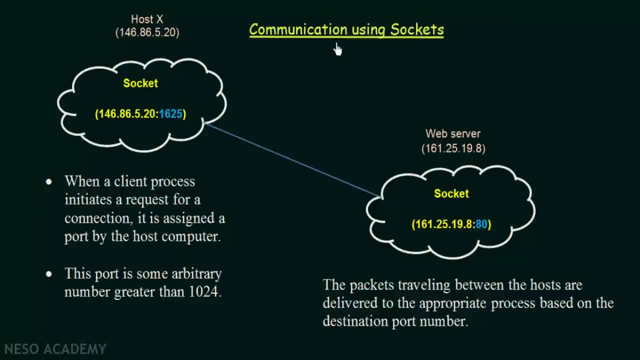 Now moving on, let us take a visual example and see how does communication using sockets takes place. So here in this diagram, I have this first part, which is the host, And I have this second part, which is the web server. Think of this as the client and this as the server. 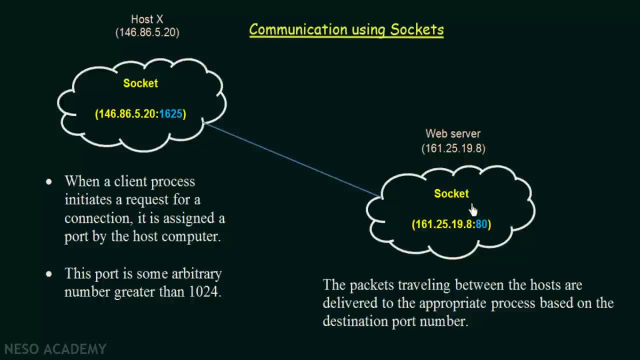 So the client wants to request something from the server And the server has to fulfill that request by giving whatever the client asks from the server. So in order for that to occur, we need to have a communication link between this server and the client. 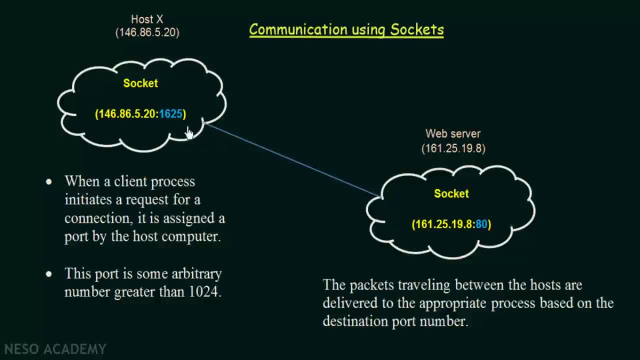 There has to be some kind of link between the server and client. So, in order to establish this communication link, we are going to use the concept of sockets, which we have just studied. So let us see, This is the socket that belongs to the client. 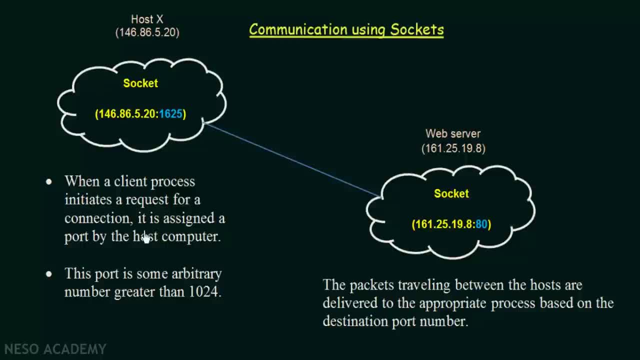 So when a client process initiates a request for connection, it is assigned a port by the host computer. So here a client process is trying to establish a connection between the client and the server. So what will happen? The host computer will assign a port number to this process which wants to communicate to the server. 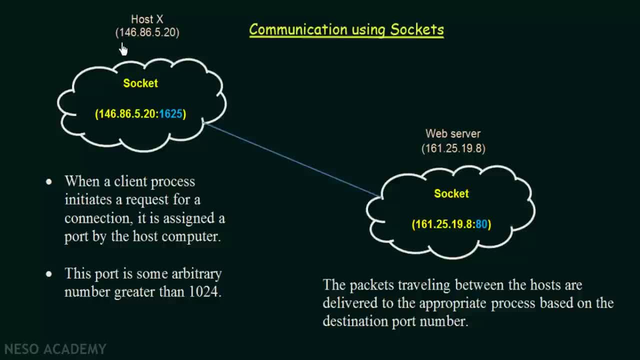 So, if you look at this, this is the IP address of the host computer, 146.86.5.20, And a process that belongs to this host computer wants to communicate to the web server. So what will happen? A specific port number will be assigned by the host computer to this client process. 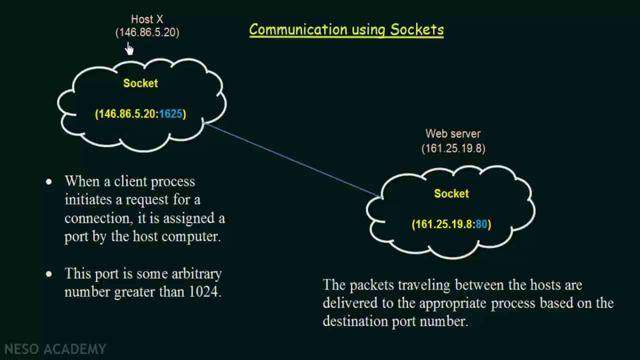 So, if you look at this, this is the IP address, which is same as the IP address of the host, And it is concatenated with a port number. So, as I told you, sockets are identified by an IP address followed by a port number. 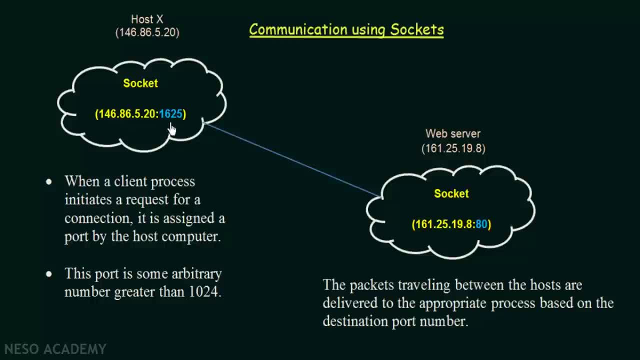 So this first part is the IP address and this second part is the port number. So this port number is some arbitrary number greater than 1024.. And why should it be greater than 1024? Because the port numbers below 1024 are considered well known and are used for implementing standard services. 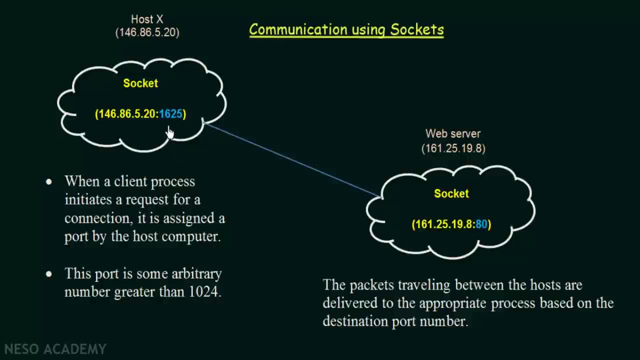 We have already seen that. So whenever a port number is assigned to the process, it has to be something greater than 1024.. Like, for example, here we have used 1625.. So here the socket is established, And similarly in the web server. 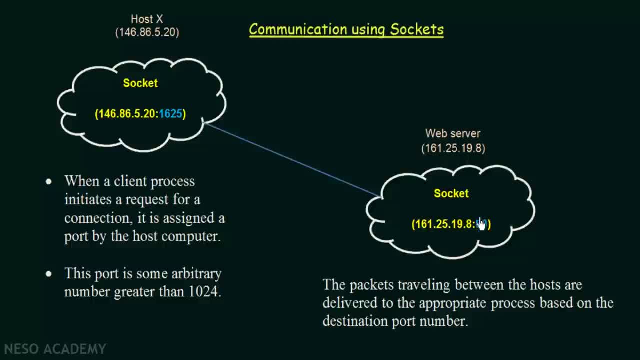 here this is the IP address of the web server, And this web server also has a socket, And that socket belongs to the process in the web server that is going to communicate with this client process. So here also we see this IP address is same as that of the web server. 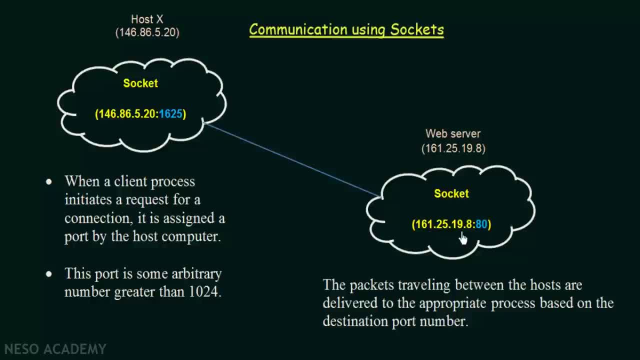 And here we have port number 80 assigned here, And when you look at port number 80, you will see that port number 80 is assigned here. So if you look at port number 80, you will know that it is less than 1024. 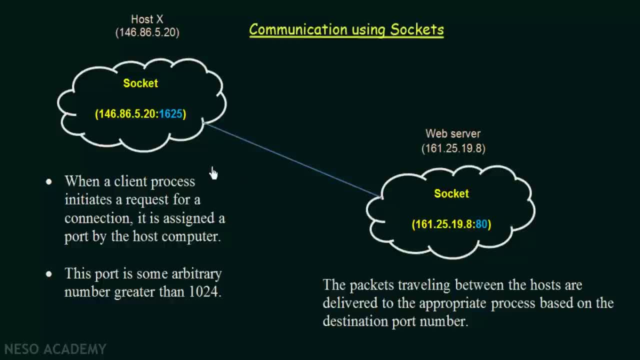 That is because this is the server, not the client. So this client is trying to access some server. So the port number 80 belongs to some standard services which is there And this client process is trying to access that. So the packets travelling between the host. 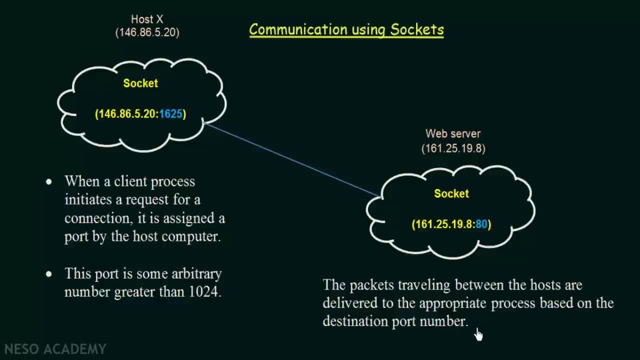 are delivered to the appropriate process based on the destination port number. So the packets that are traveling from this client process, from this client process to the server process, are delivered appropriately based on the port numbers. So here there is a standard service with port number 80.